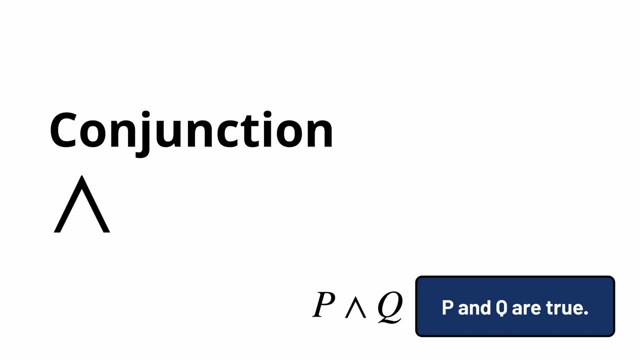 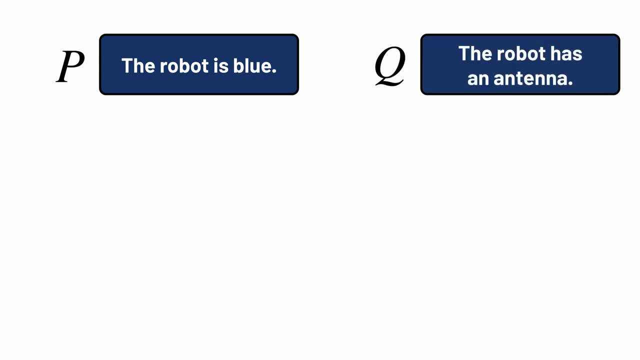 formulas and expresses the idea that both are true. So if p is the proposition the robot is blue and q is the proposition the robot has an antenna, then the conjunction p and q is a formula that's true when the robot in question is both blue and has an antenna as well. 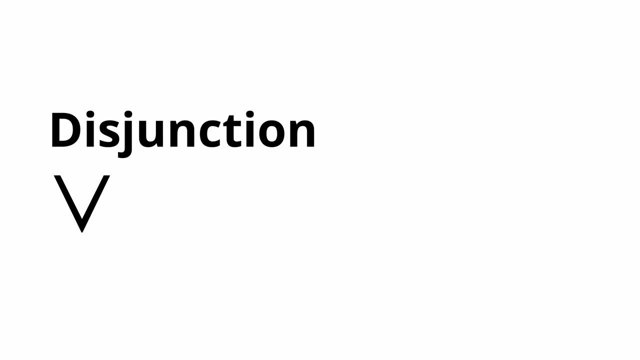 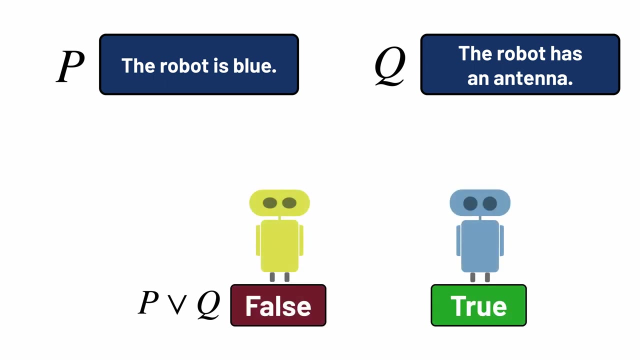 Meanwhile, this symbol called disjunction or or takes two logical formulas and expresses the idea that at least one of them is true. In this case, the disjunction p or q is a formula that's true as long as the robot is blue or has an antenna, or maybe both, Especially once we start dealing with 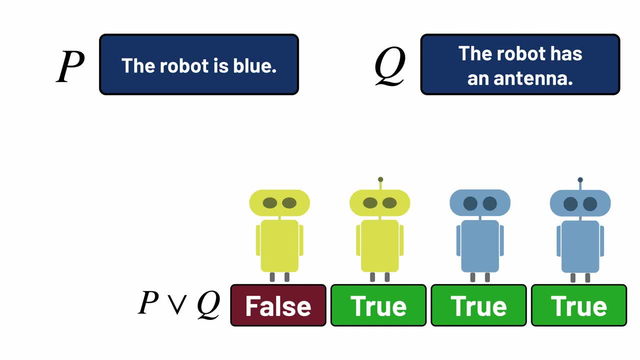 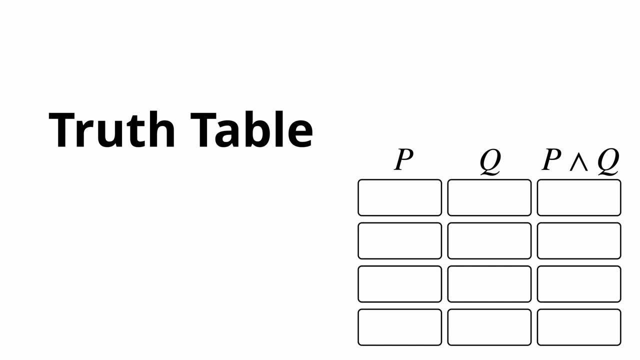 multiple logical variables in a formula, it can be useful to figure out under what circumstances the formula is true and under what circumstances the formula is false. To do that, we can create a truth table, a table that lists all of the possible combinations. of values for the logical variables in a formula and what the means for the familiar side of the formula. In this case you can differentiate the two variables p and q, so two причines would be both false and true. To immediately solve the problem, you need to write for me the list of possible combinations. of values for the logical variables in a formula To finally means for whether the formula is true or false and then apply p tomorrow. There are four possible combinations of values for the logical variables in a formula. In the previous document we learned that the three variables are possible. 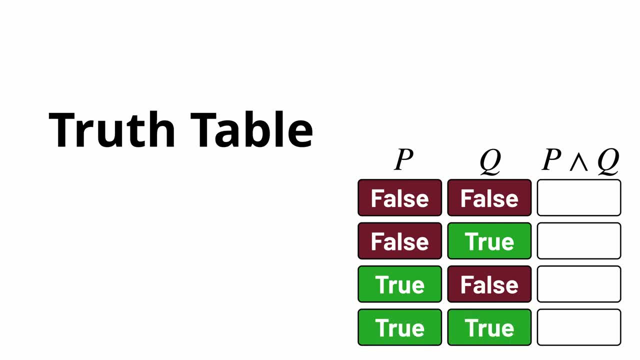 Here we alcohol, AGod beiä. and P and hq are both the real variables. These two are possible combinations of values. for the logical variables be true while q is false, or both could be true. For the formula p and q, there's only one setting. 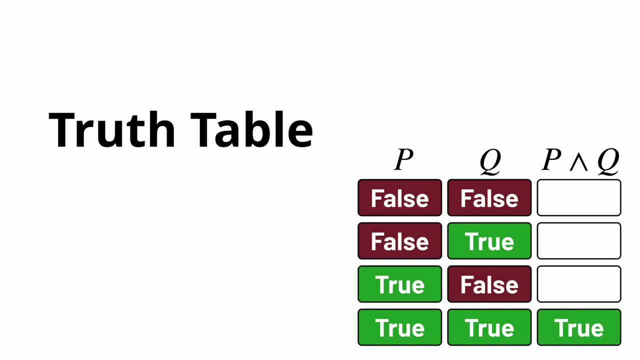 of these variables where it holds true. p needs to be true and q needs to be true as well. In all other cases, the formula p and q is false. But for the formula p or q, three of the four combinations of values allow the formula as a whole to hold true, and only in the case where p and q are both. 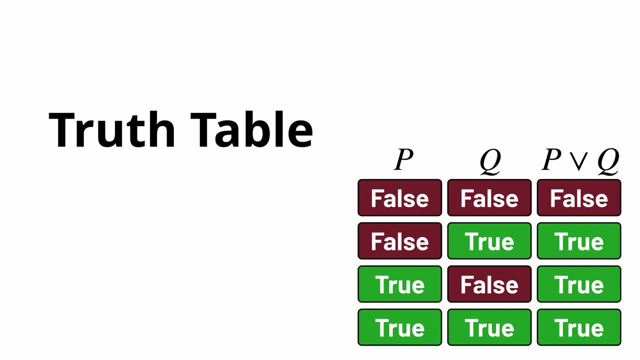 false, is the formula false. Notice that for the formula p or q, it's true if p is true or if q is true, or if both are true. Sometimes, though, we'll want to express the idea that p is true or q is true, but not both. For that we can use. 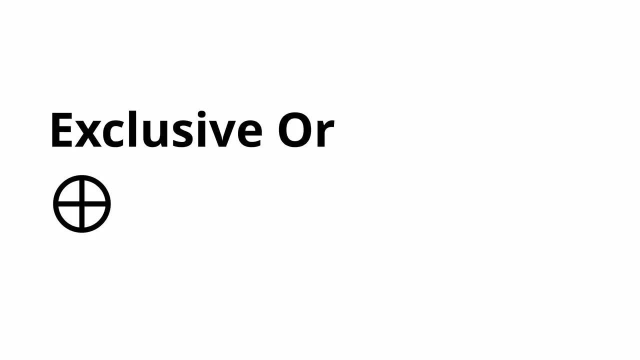 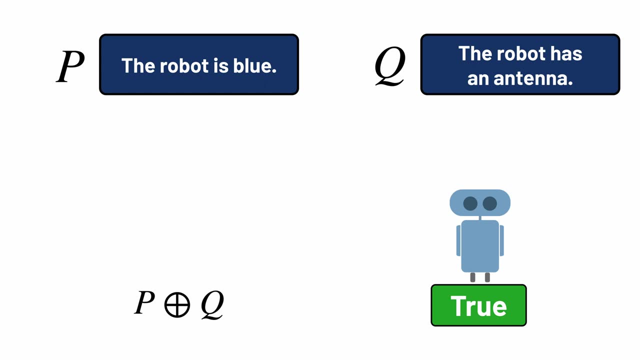 this symbol, called exclusiveOr, In this case, p, exclusiveOr q, is true when the robot is blue, it's true when the robot has an antenna. it's false when the robot is not blue and doesn't have an antenna, and it's also false when the robot is both blue and has an antenna. 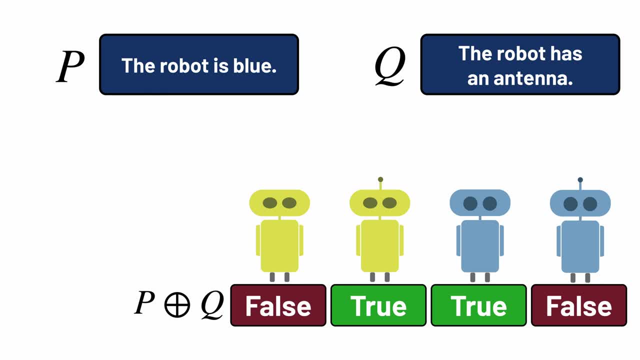 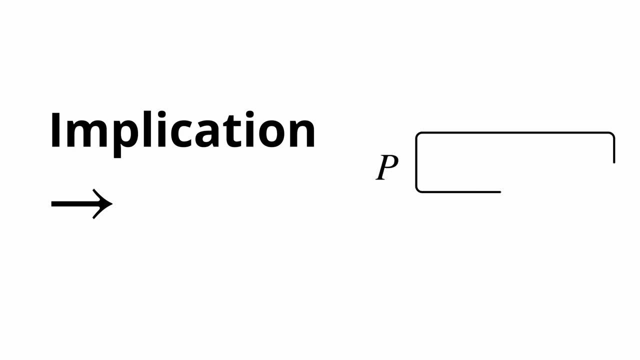 In addition to not and or and exclusiveOr, we also have this symbol called logical implication. If p means the robot is blue and q means the robot has an antenna, then this formula, which we read as p, implies q. or alternatively, if p then q. 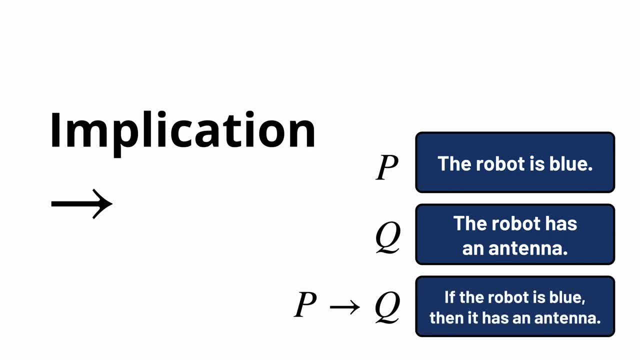 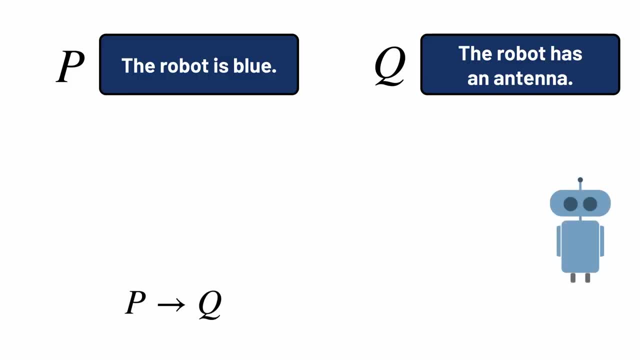 tells us that if it's true that the robot is blue, then it also must be true that the robot has an antenna. So for this robot it's blue and it has an antenna. so p implies q is true. But for this robot it's blue, but it has no antenna. 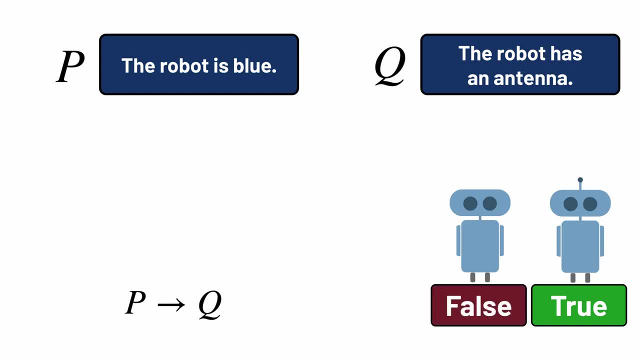 so p implies q is false here. For it to be true, the fact that the robot is blue would have to imply that the robot has an antenna. Importantly, p implies q says nothing about what the world must be like if p is false. If p is false, in other words, if the robot isn't blue, 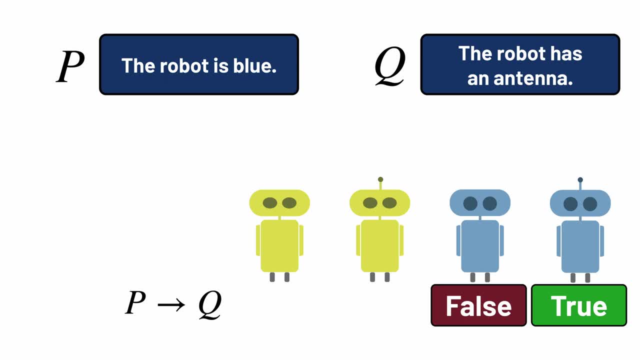 then the formula isn't saying anything about whether q is true or not. Maybe the robot has an antenna, maybe it doesn't. In either case, p implies q is true. It can be a little tricky to wrap your mind around the idea that p implies q is true in all cases where p is false. 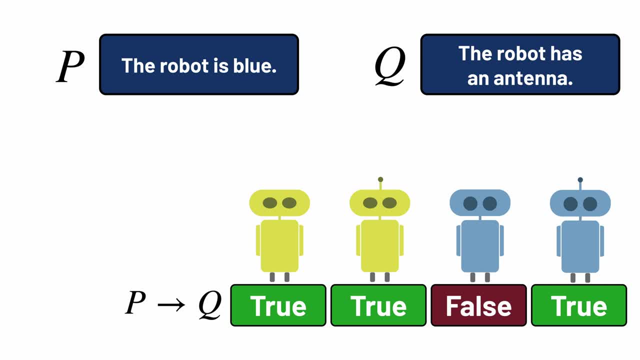 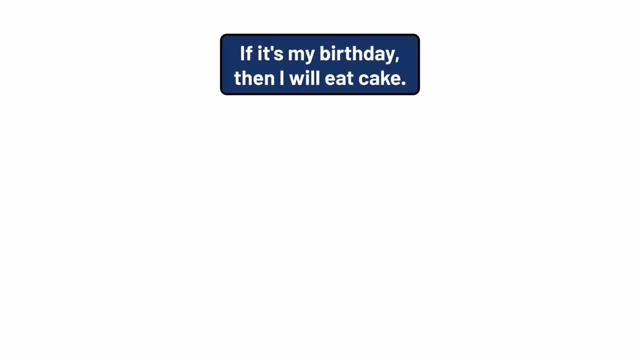 But this fits logically with how we use the ideas of if and then in everyday life. For example, imagine you said something like: if it's my birthday, then I will eat cake. For that to be true, then on your birthday you need to eat cake, but on days where it's not your birthday 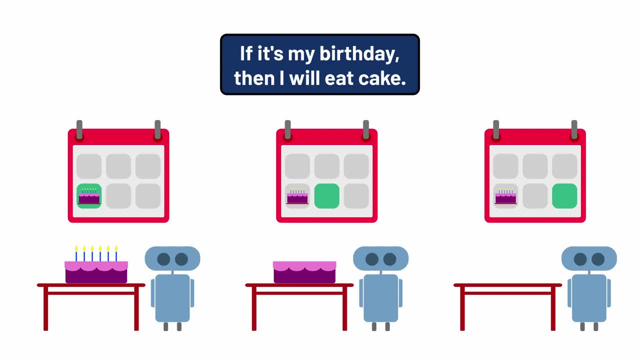 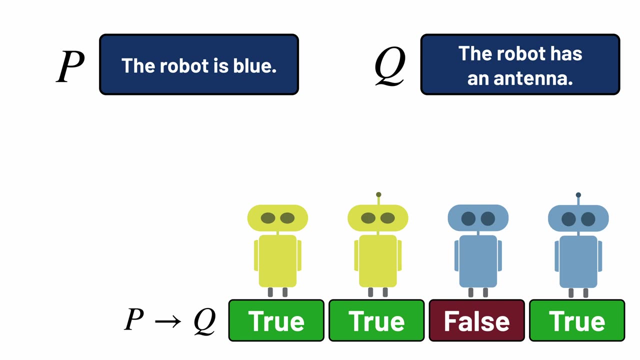 you might eat cake or you might not, and you could still be telling the truth. The only way you wouldn't be telling the truth is if it's your birthday but you don't eat cake. So let's go back to blue robots and antennas. The formula p implies q is true. if p implies q is true. 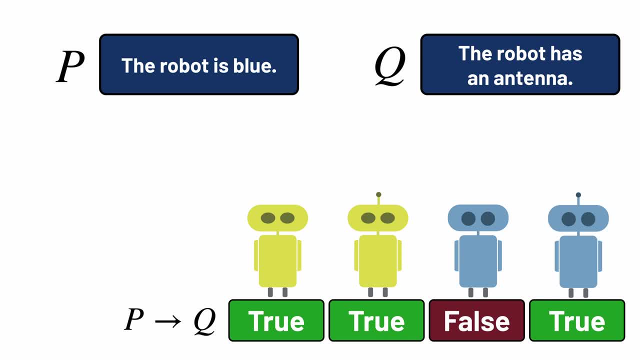 for a blue robot with an antenna, and it's true for any robot that isn't blue. So there's another way to express this same idea, too. We could equivalently say not p or q, which is true when the robot isn't blue or when the robot has an antenna. 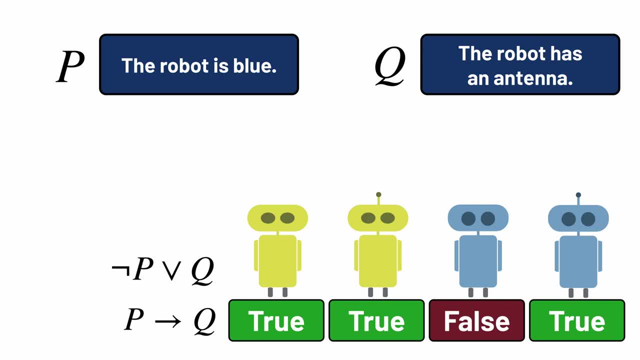 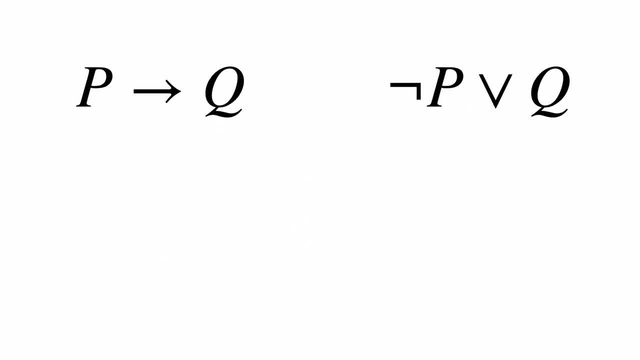 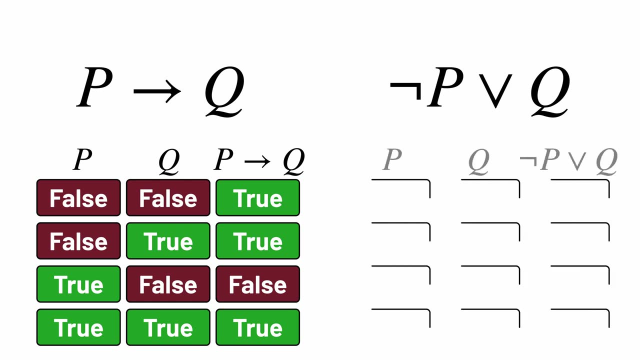 In other words, these two formulas are logically equivalent to each other and we can prove that by writing out the truth tables for each formula. We can describe the situations where p implies q is true and describe the situations where not p or q is true And it turns out the truth tables are: 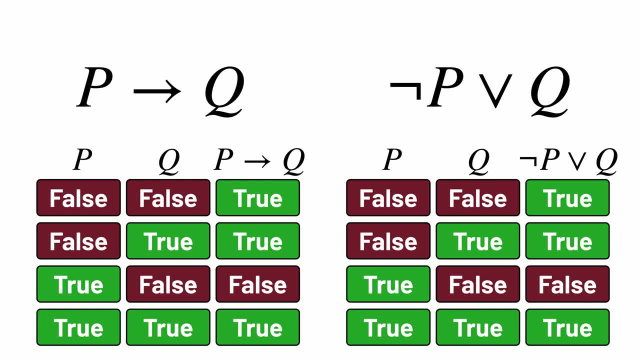 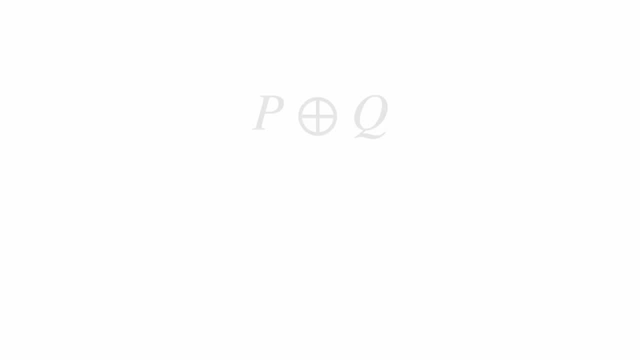 the same. No matter what the values are for these variables, p and q, these two logical formulas will always have the same truth value. Many logical formulas are equivalent to each other. For example, you might try on your own proving that p exclusive or q means the. 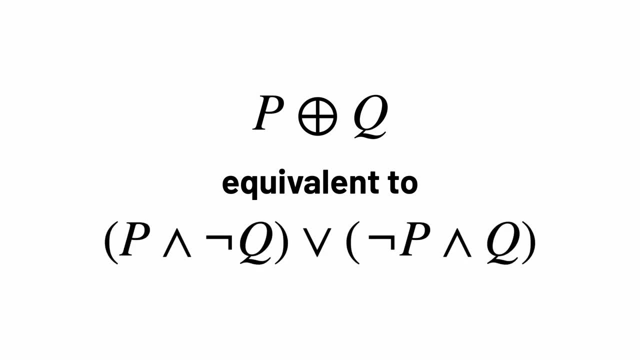 same thing as p and not q, or not p and q, And you can try on your own to find other logical formulas that are equivalent to both of these two. Here's an exercise we can try together: Is p implies q equivalent to q implies p? We can answer that by drawing out the truth. 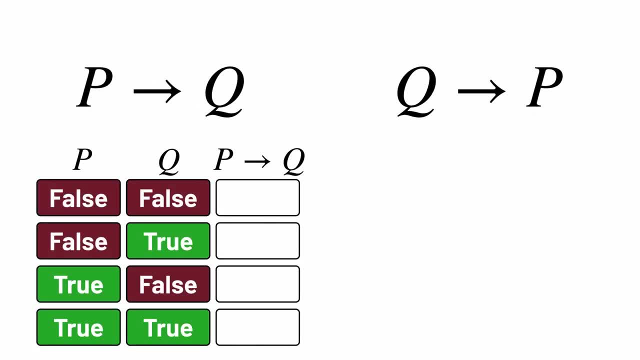 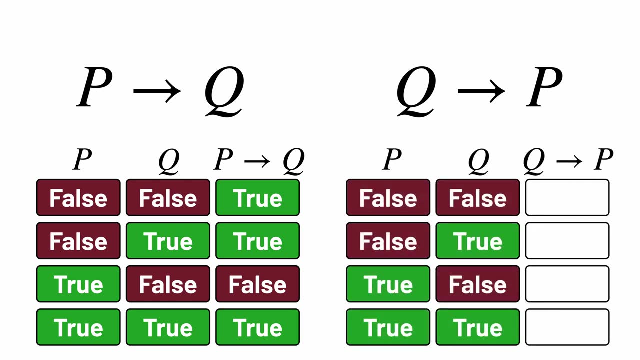 table: p implies q means that if p is true, then q is true. So if p is true and q is false, then the whole formula is false. And if p is false, we know the formula is true, no matter what Meanwhile. q implies p means that if q is true, then p is true, And when q is false, 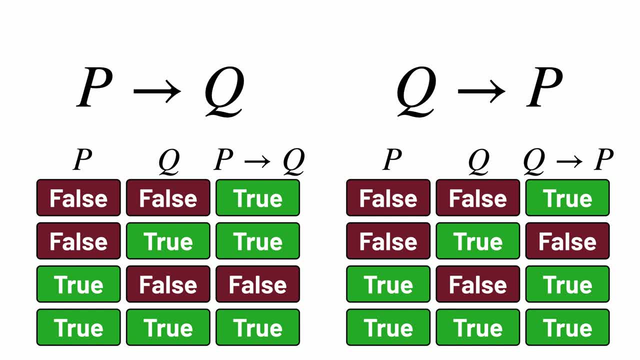 the formula again is always true. Notice that these two truth tables are different. So p implies q and q implies p mean two different things, And that makes sense too, given how we intuitively think about if and then. When I say if it's a holiday, then the bank is.